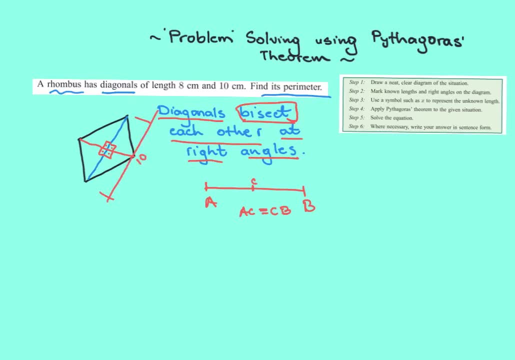 like that. Okay, So that one is 10 and this one here we're going to say it's equal to 8, because that's the given And diagonals are bisected. So we do know now that this part here, now we look straight down and 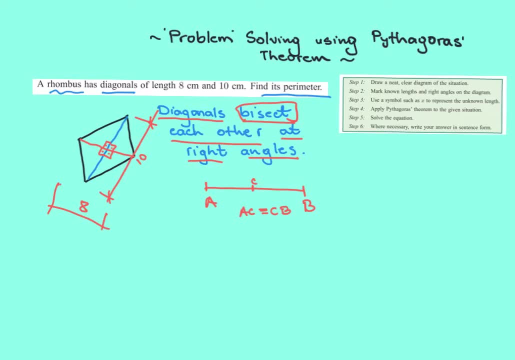 that this right here will now become the diagonal, because diagonals are bisected. so we do know now that this part here, from this corner to here, it is equal to 4.. I'm going to put 4 here and I'm going to put 4 there. 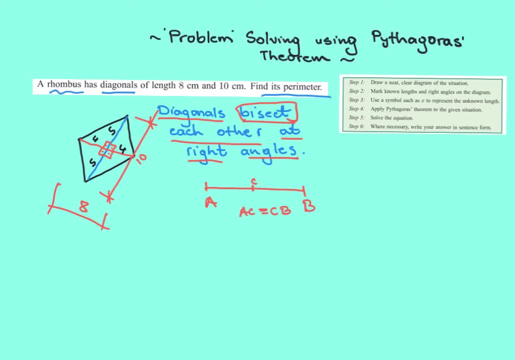 So I picked 4 here instead of 5, because this diagonal second half is five as well. now if you just focus on um one part of the rhombus which is this one here. so i'm gonna take this uh picture out, so i'm gonna draw a picture. 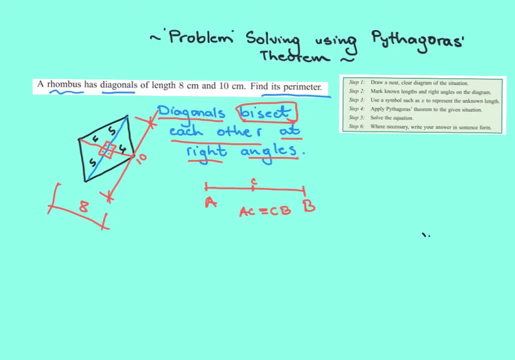 um, it's gonna look like this: let's move here. so that's this one. so we have right angle here. and this is five, and this is four. maybe i'm gonna use the same colors, just to know what i'm talking about. uh, not that you don't know, but um, and this one here. okay, so now we do have right. 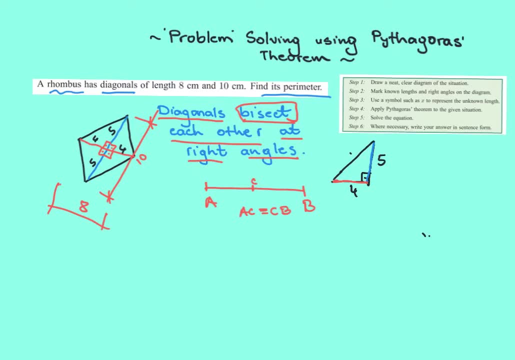 angle triangle. so, and in order to find the perimeter- i should have said that before- in order to find the perimeter, we need the length of all these sides. okay, so all these sides. so we do know that they're, all sides are um equal anyway, but we don't know that. 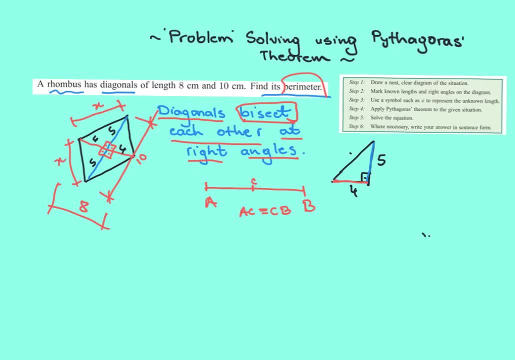 so we're gonna label x. that's usually is x, y, z, but you can use any letter you want, so and those letters are called variables, by the way. so let's have a look at this one here: x. so according to pythagoras theory, so x is a cross right angle and it's the longest side of the triangle, and 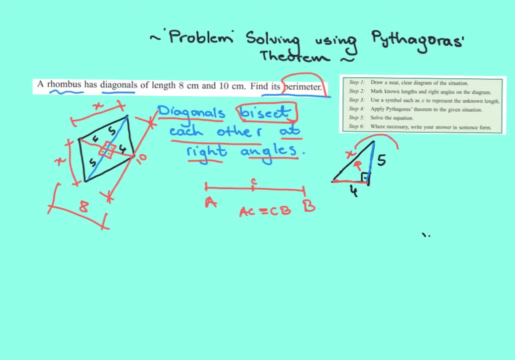 hypotenuse, by the way. so like i'm just gonna go here, hypotenuse okay, and it's the longest side. so how are we gonna calculate? so x to the power of 2 is equal to 5 to the power of 2 plus 4 to. 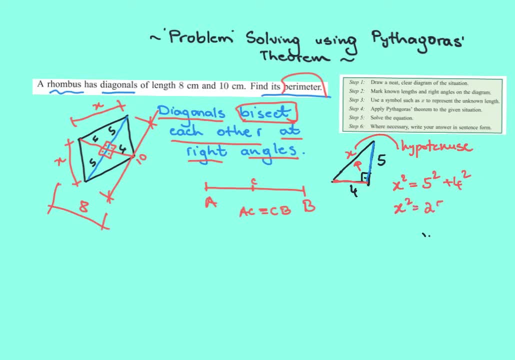 the power of 2. x to the power of 2 is equal 25 plus 16, and then x to the power of 2 is equal to 1, and as now we have x to the power of 2, we want x by itself, and i'm gonna find the square root of. 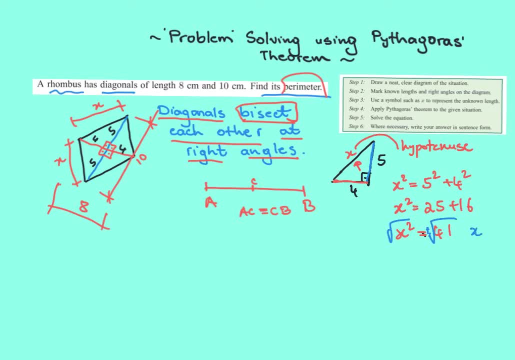 both sides. and i'm gonna say here: x is bigger than zero, as we are talking about the length, so we're not gonna have negative one. so therefore x is equal, only positive square root of one. so now what do we need to find perimeter? yeah, it's just here. so that is the question. 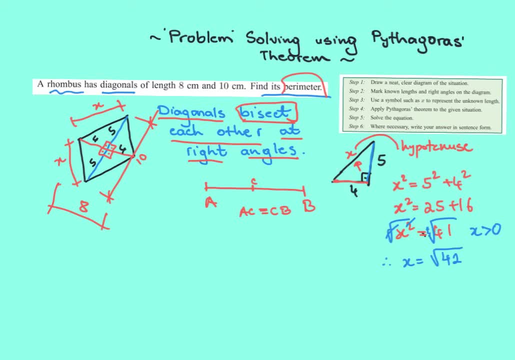 perimeter. so how are we gonna find perimeter? perimeter is adding all sides, so therefore yellow, how it does look like. no, i'm gonna go back to um black. so therefore perimeter is 4 times 4 sides of, so 4. okay, i'm gonna go to 4 sides of square root of 42 and we know. 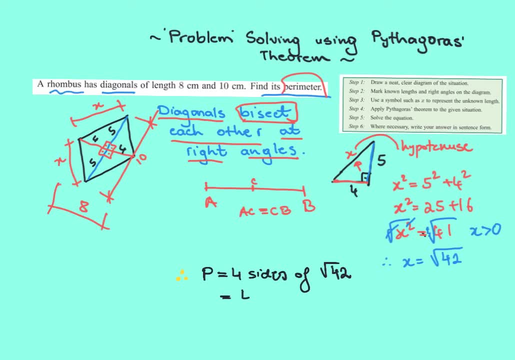 off in maths is multiplication, so 4 times square root of 42. now, um, if you're in building industry or architecture or something like that. so usually you don't say like perimeter is 4 times square root of 42, right? so you don't say like perimeter is 4 times square root of 42, right? so you don't say 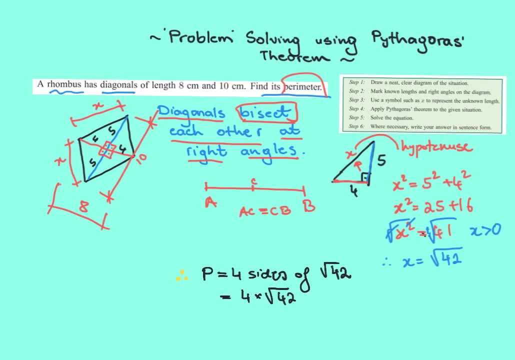 where did i get 42 from? okay, let's have a look. so, um, i have to erase. 25 plus 16 is 41. and yeah, let's have a look at this one here. this one looks like. looks like um, two. i'm gonna make adjustments there.